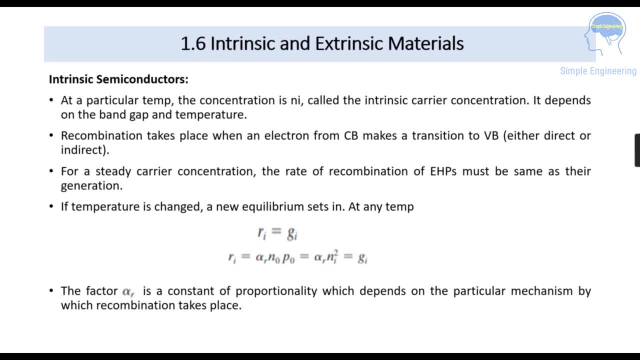 and it depends on the bandgap and temperature And the recombination that takes place when an electron from the conduction band makes a transition to the valence band. It can be either a direct transition or an indirect transition And for a steady carrier concentration, the rate of 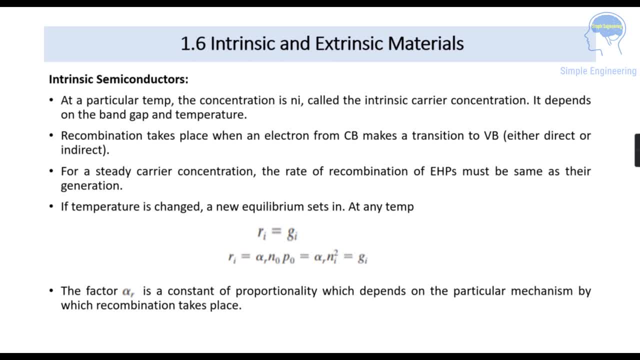 recombination of the electron hall pairs created must be the same as their generation. So if the temperature is changed, a new equilibrium is set and at any temperature the electron hall pairs in issuinged into the Java Tangoött-N해주er. Let us say that the field temperature is set. 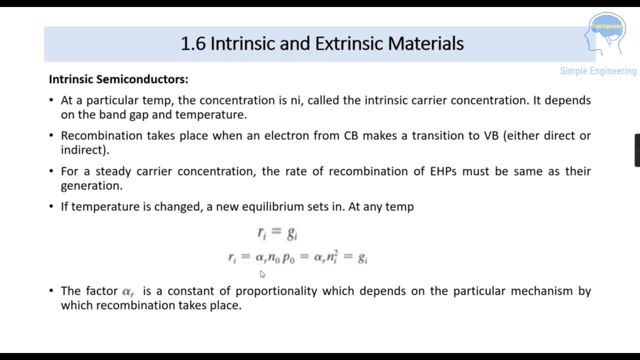 at an是這樣 temperature. this is the Won 61 degree centigradeiencia average. Thus the될 When the temperature changes from just the range at which the electron goes from. Yes, there is a scale that can be drawn along, So watt sair can come out with any frequency. 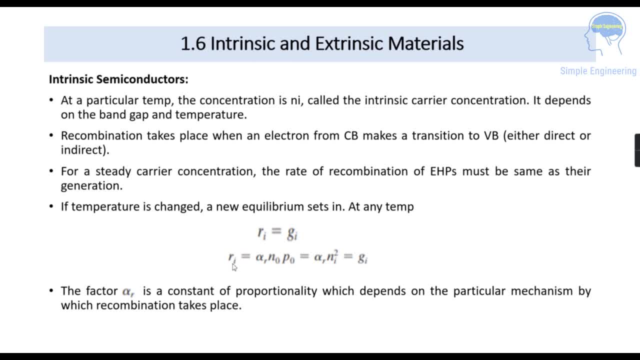 from the control band, the air flow rate can be drawn and the temperature changes as the temperature is set, partido for the rate of recombination. Here如果 hiệnي data licensure generation rate. The factor alpha r is a constant of proportionality which depends on the particular 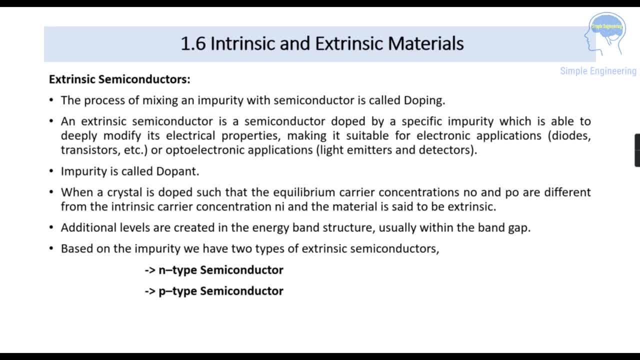 mechanism by which this recombination takes place. Next is extrinsic semiconductor. Here we are mixing an impurity with that semiconductor. That mixing of impurity is called doping. So an impurity is doped into the semiconductor. So by doping a special impurity, it will modify its. 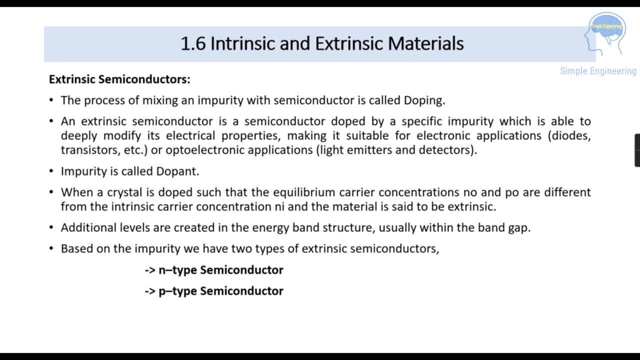 electrical properties and it will make that material, or it is making it suitable for the electronic application or some optoelectronic applications, And we are adding the impurity to that semiconductor that is called a doping. So when a crystal is doped such that its equilibrium 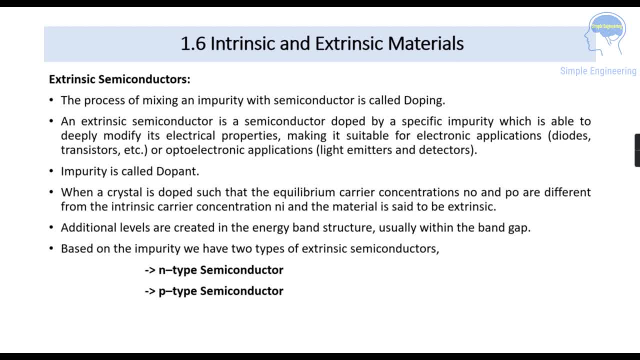 carrier concentration N0 and P0 are different from the intrinsic carrier concentration Ni, And that material is said to be an extrinsic semiconductor And additional levels are created in the energy band structure, usually within that band gap And based on the impurity that we are adding. 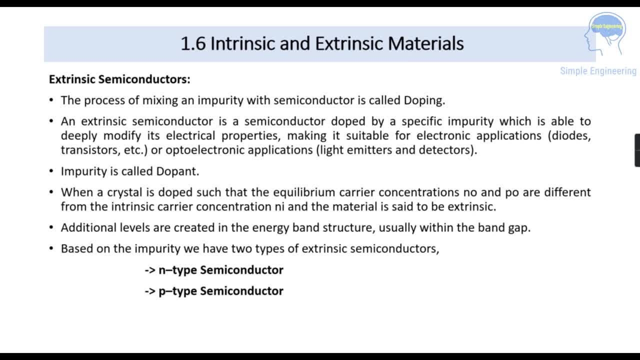 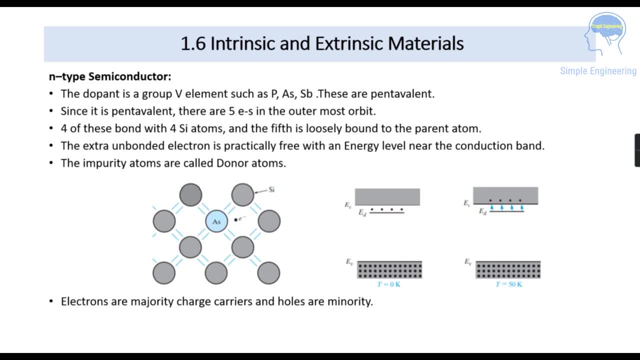 to the semiconductor. this extrinsic semiconductor is classified into two types: p-type semiconductor and n-type semiconductor. So first we will see about n-type semiconductor. So in this extrinsic semiconductor we are adding an impurity. So impurity can be, or it is, the doping It is of. if we are taking group five elements such as: 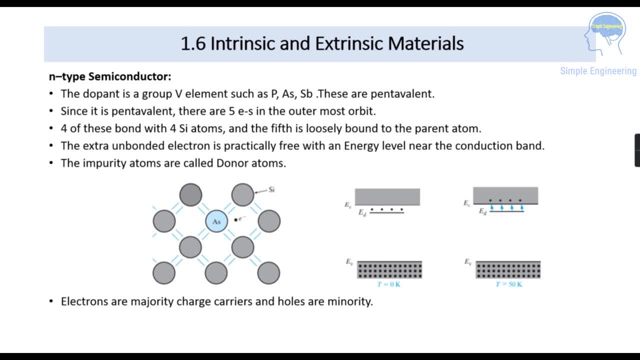 phosphorus and arsenic means it is called n-type semiconductor because it is a pentavalent doping. So pentavalent means, in that doping which we are adding, or that element, phosphorus or arsenic, it will be having five electrons in the outermost orbit, So four of these will be in a bond with the. 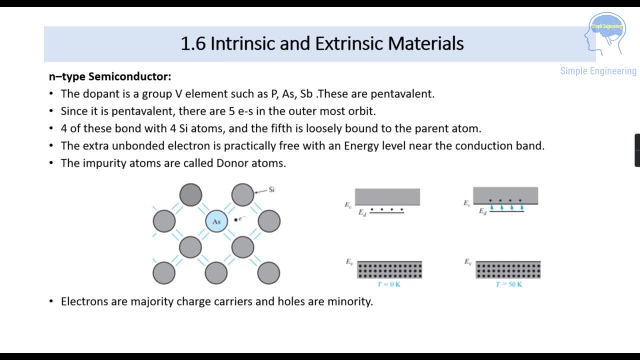 silicon atoms, and the fifth one will be loosely bound, So that extra unbounded electron that is free to move within that energy level near the conduction band and the impurity atoms are called donor atoms. So in this figure you can see that arsenic, the blue color one, which is a. 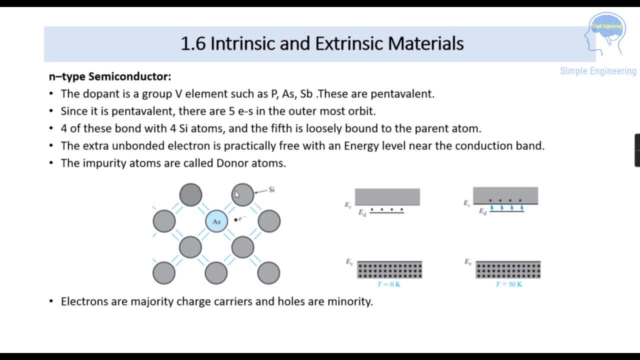 pentavalent doping which we are adding into that semiconductor. So silicon atoms are surrounded by them. Silicon is this will be in a bond with the arsenic, where arsenic is having five electrons in the balance band and silicon is having four. So 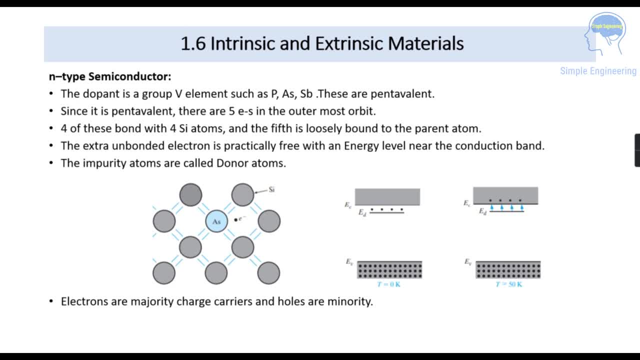 it will be in a bond with the four atoms and the fifth one will be free. So when the temperature is at zero Kelvin, you can see that this is the valence band and this is the conduction band, and here this is your donor atoms. So these atoms will excite to the conduction band when your 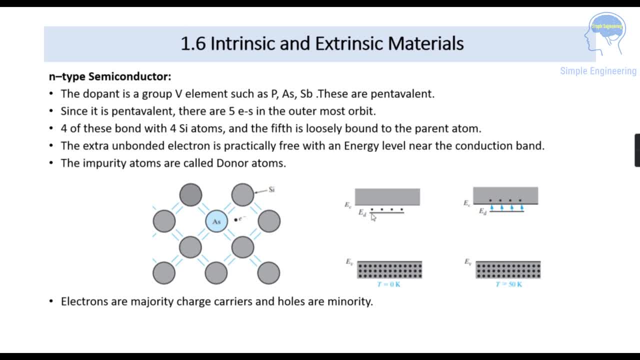 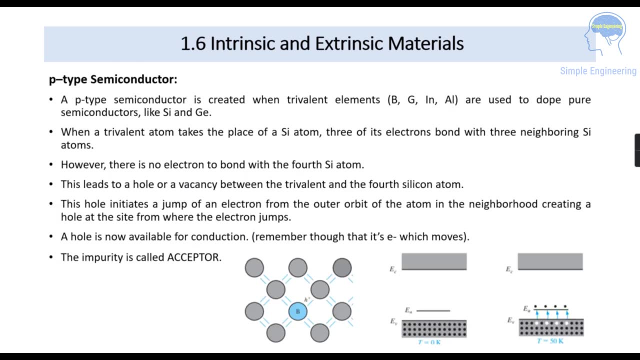 temperature starts increasing. That temperature is equal to zero. you can see that the donor atoms is in this energy level. When your temperature is at 50 Kelvin, it will excite to the conduction band. So the electrons are the majority carriers and the holes are the minority carriers here. Next is P. 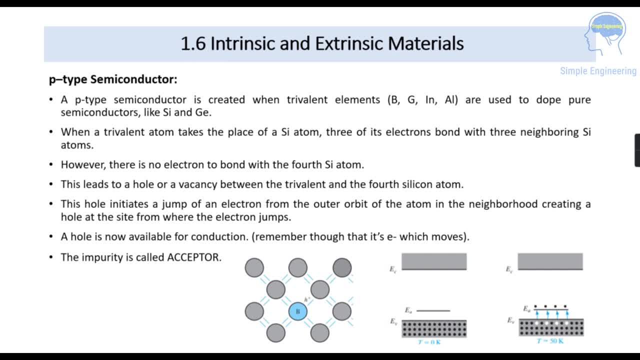 type semiconductor. So in N type semiconductor we are adding the pentavalent impurity. So in P type semiconductor we are adding a trivalent element such as boron, indium and aluminium and silicon and this will be in a bond with the silicon atom. So in this figure you can see that. 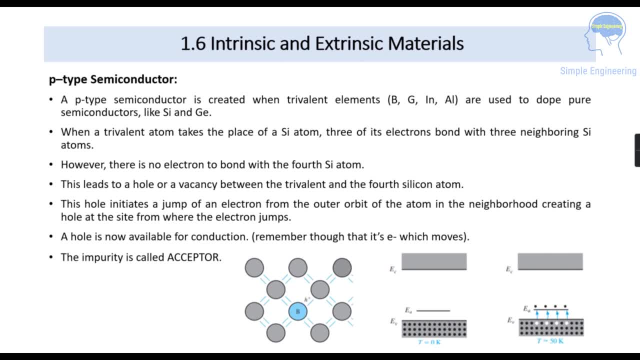 boron, which is having only three electrons in the outer core, So it will be in a bond with the silicon atoms. but silicon is having four electrons So there will be a one fourth silicon atom. It is there is no electron to bond with that, So this leads to a hole or a vacant, vacant portion in the 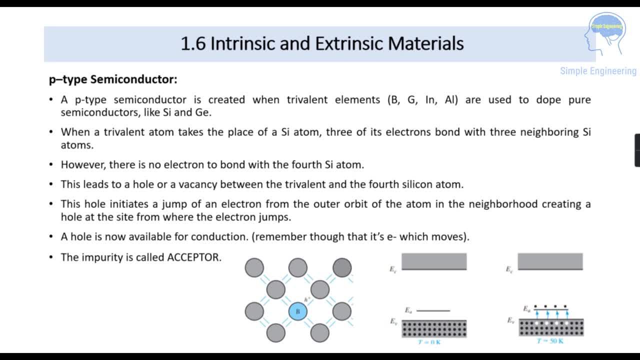 between that trivalent and the fourth silicon atom hall. it initiate a jump of an electron from the outer orbit of the atom and the hall is now available for conduction. and the impurity which we are adding here in the p-type semiconductor is called acceptor. So in the figure you can see that when the temperature is 0 kelvin you have 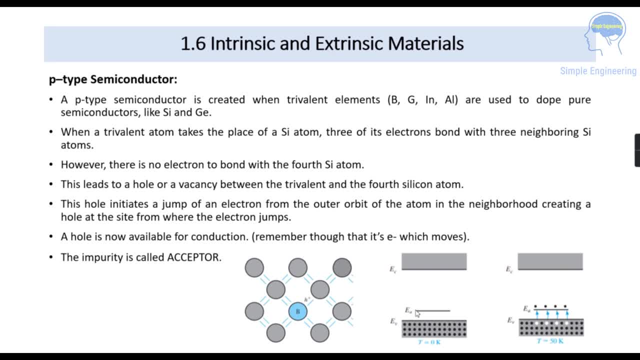 electrons in the valence band and this is your acceptor level and this is your conduction band. When the temperature starts increasing, the electrons in the in your valence band it will be in the, that is the impurity acceptor atoms. So here vacant space will be created. that is the halls. 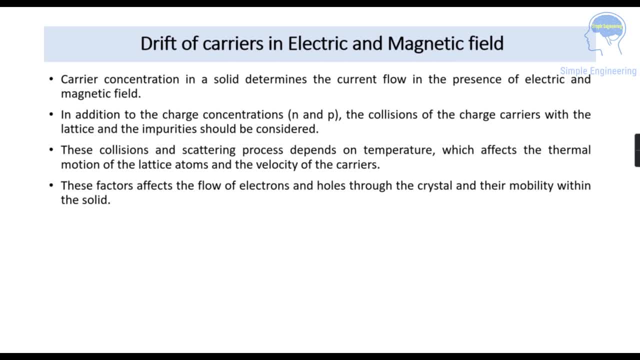 Then next is the drift of carriers in the electric and magnetic field. So how that carrier drift is happening, So carrier concentration in a solid that determines the current current, the current flow in the presence of an electric and magnetic field. so in addition to the charge, 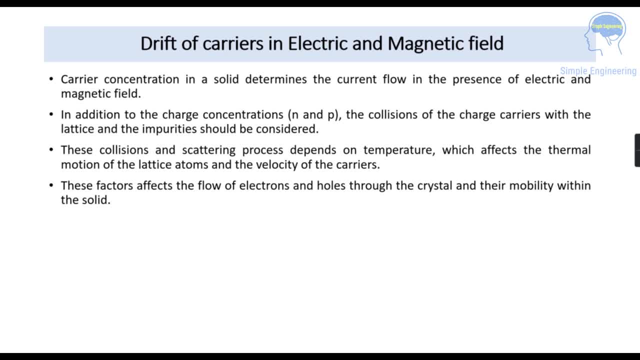 concentrations, that is, your electrons and holes n and p, there will be the collision of that charge carriers with the lattice and the impurities should be considered. so these collisions and scattering process it depends on the temperature which affect the thermal motion of that lattice atoms and the velocity of the carriers, and these factors affect the flow of electrons and holes. 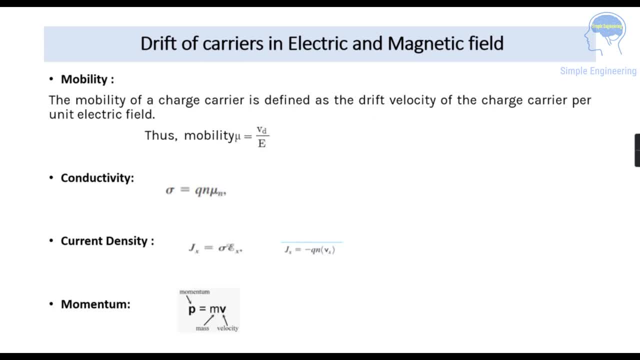 through the crystal and their mobility within that solid. next is the terms which we have to consider. that is mobility, which means it is, it is denoted as mu, it is equal to vd by e, where vd is the drift velocity and e is the electric field. so mobility of the charge carrier means it is defined as the drift velocity of that charge.